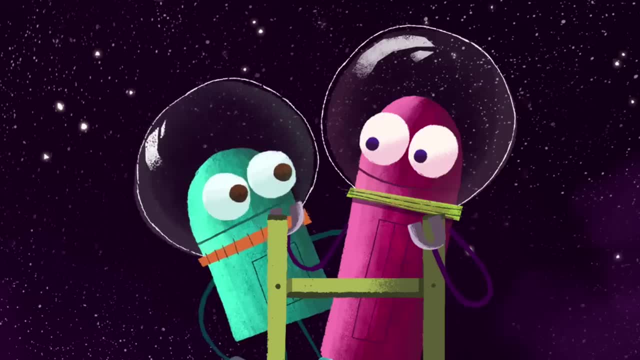 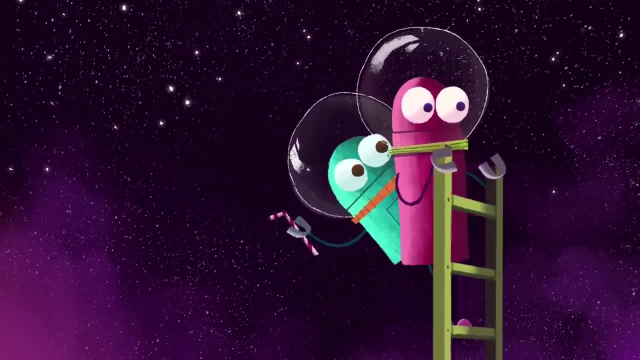 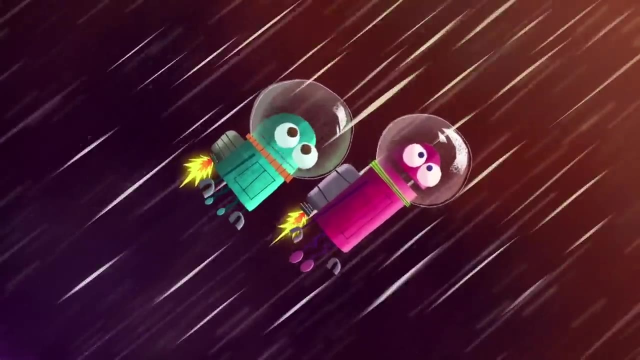 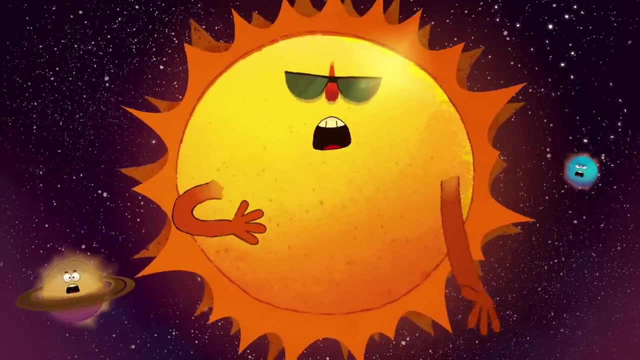 Well, we are done exploring the solar system. I am thirsty. Let's explore the rest of the Milky Way galaxy. According to my calculations, we are now approaching the sun. It's getting pretty hot in here. I'm so hot, I'm so hot, Check me out, Check me out, I'm hot. 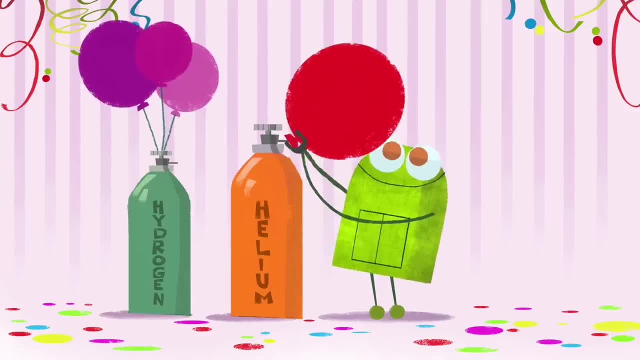 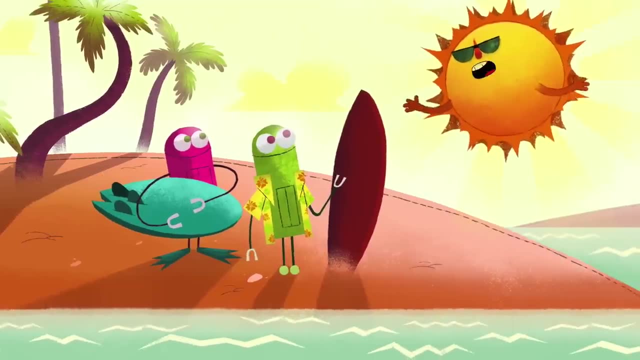 Yo everyone. I'm the sun. I'm made of gas like hydrogen and helium. I keep the earth warm and help to grow food. I shine on the beach, on guys who say I set into the west and on comes night, And then I rise from the east with that golden light. 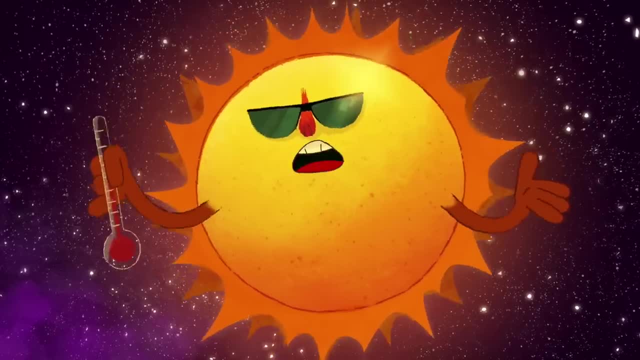 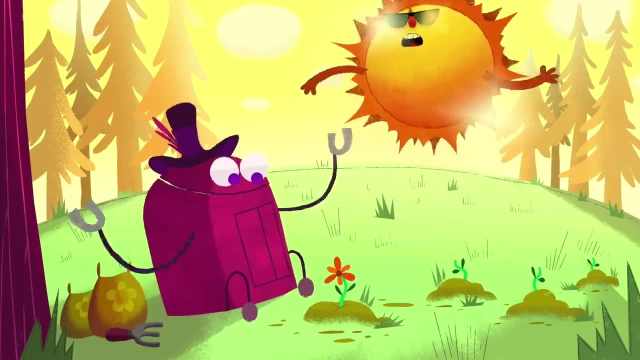 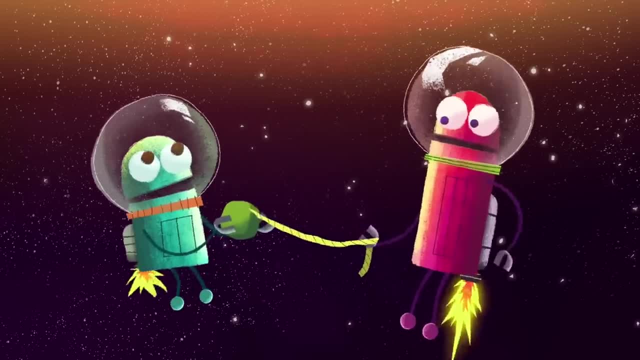 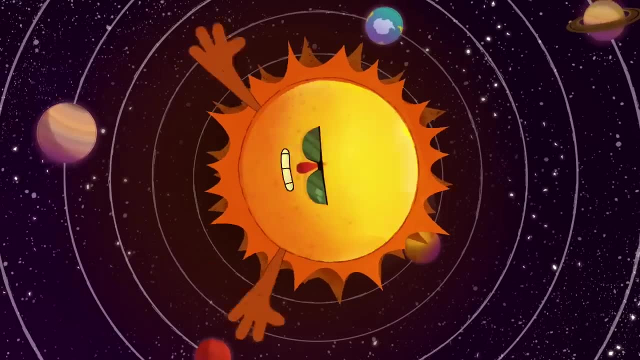 Don't stare right at me, I could hurt your eyes. I'm just about a million miles wide. I'm so big you could fit a million earths inside. I'm the center of the solar system, Can't you see? Got so much gravity. Planets orbit me. I'm four and a half billion years old. 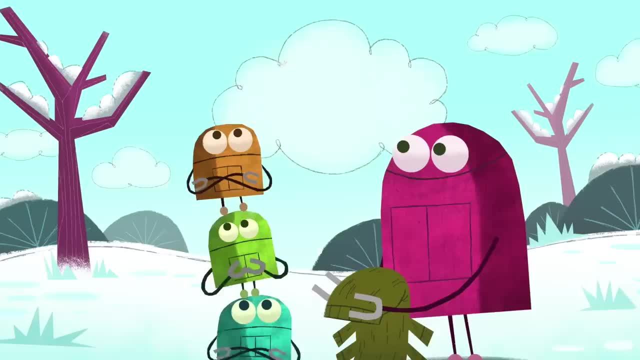 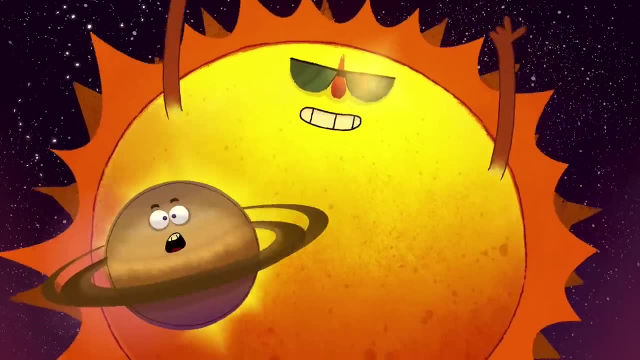 In Spanish, everybody calls me soul. When I'm not around, you'll be feeling cold. I'm so light with my rays of gold. I'm so hot, I'm so hot, I'm so hot. Oh, he's right, He's really hot. 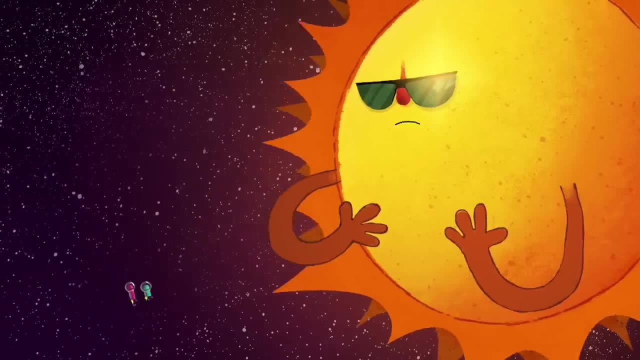 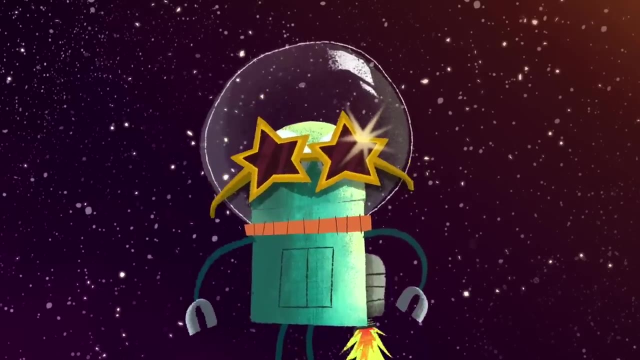 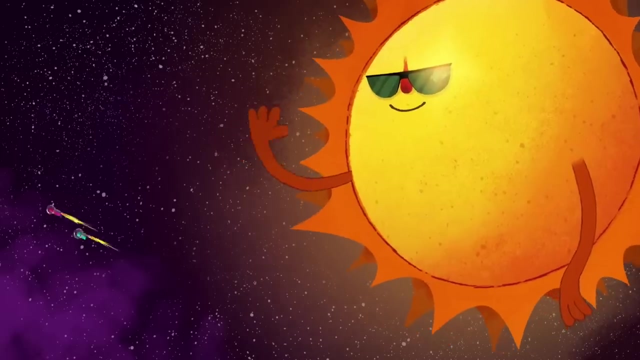 Come on, storybots, Show me what you got. How hot am I So hot? The sun is so hot. I have to wear these Now. I'm cool, So cold. I'm so hot. I'm so hot. I have to wear these Now. I'm cool, So cold. 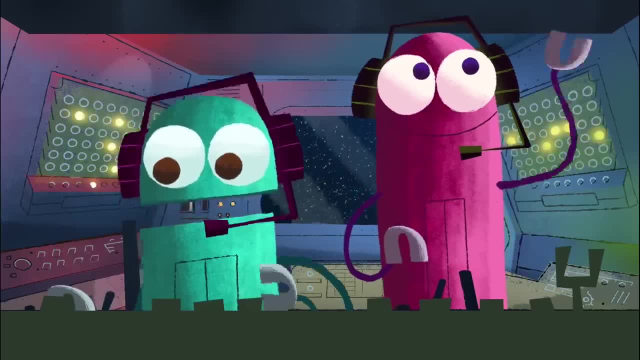 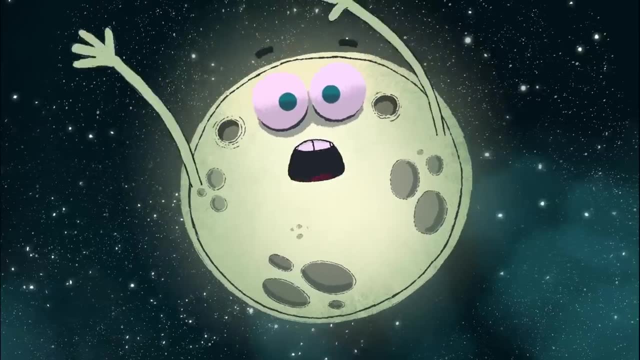 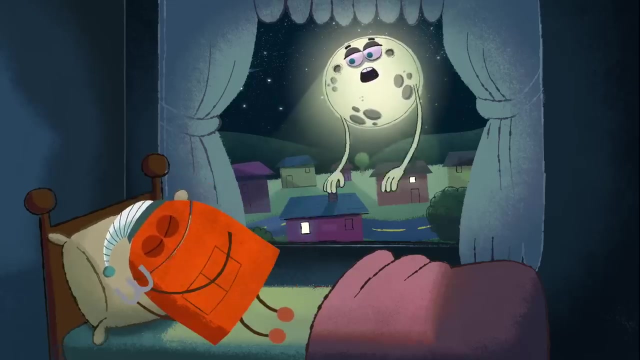 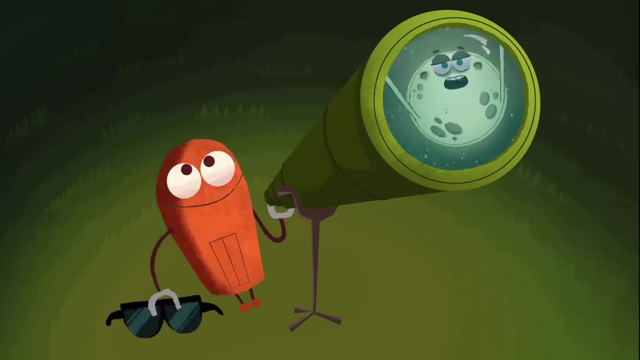 Preparing to land our spacecraft on the moon. Houston, we have a sun. It's my time to shine. It's my time to shine. The day is over now, so it's my time to shine. Good evening, it's the moon Here to regale you with a tune. I'm so bright up in the sky at night. 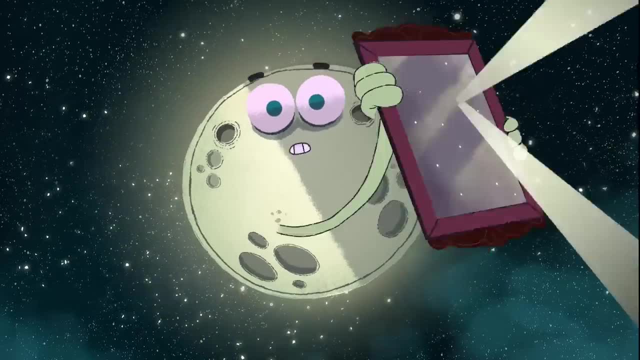 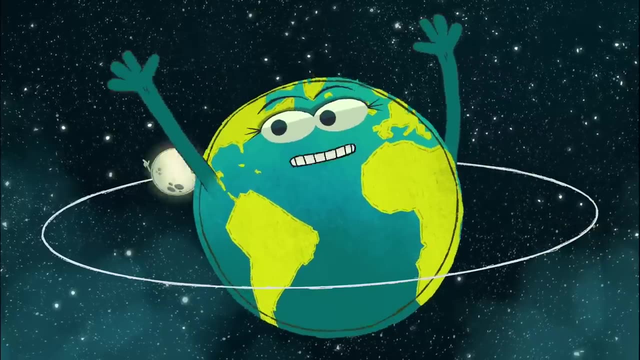 but the truth is I'm just reflecting light. See, let me help you break it down. The earth and I are spinning around and I orbit the earth in a loop. You see, the moon is kind of like my hula hoop. We both orbit the sun. He's the big shot. 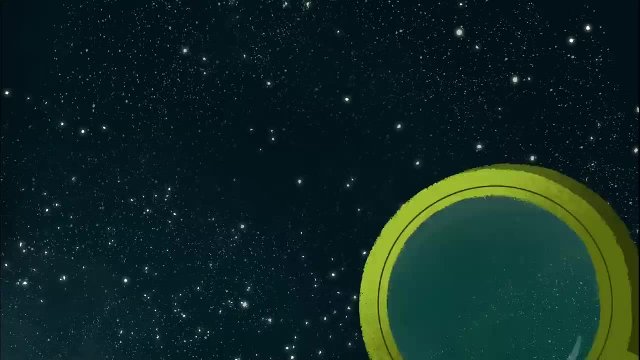 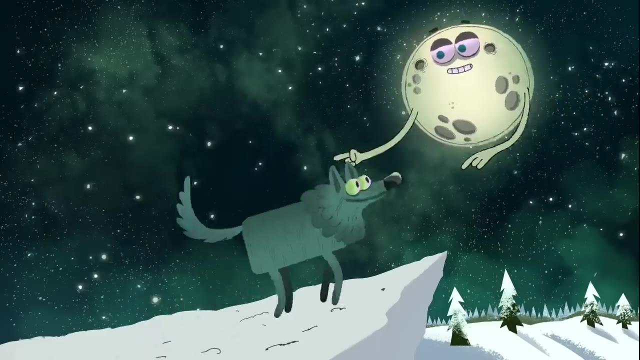 I'm the center of the solar system. I'm so hot. The sun's like a light bulb and I'm like a mirror. Light bounces off me and then it appears to the earth below for a lovely view, But animals like wolves who go awoo. Sometimes I'm full, sometimes half on. 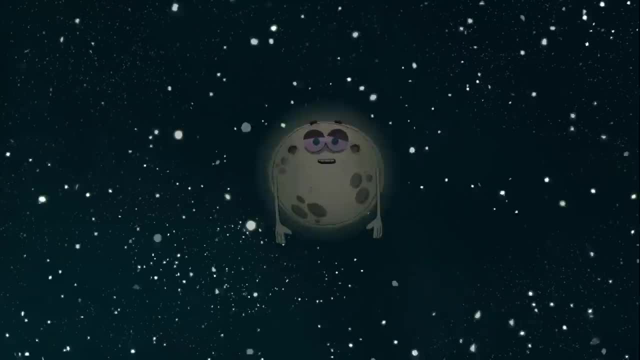 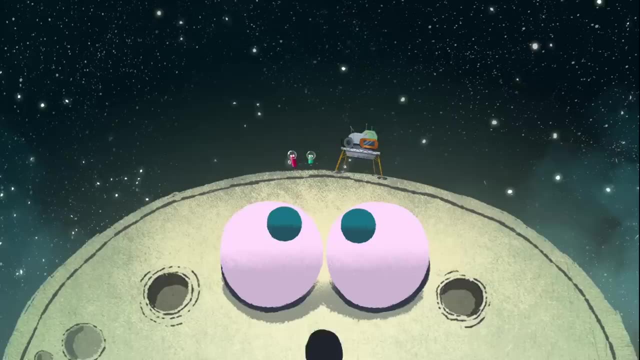 Sometimes I'm crescent or it looks like I'm gone, But I'm here in the dark, just a lonely moon, Hoping that somebody will visit me soon. I'm covered in dust and I'm made of rock, So come see me soon and go on a moonwalk. 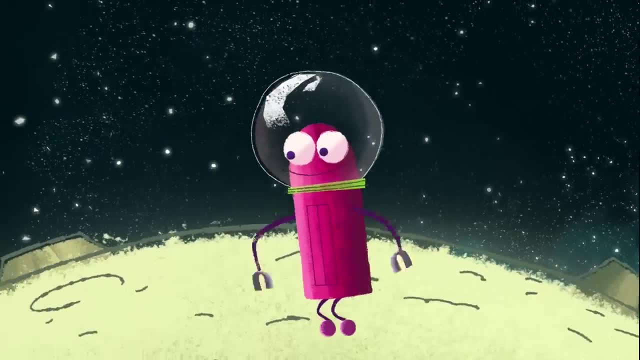 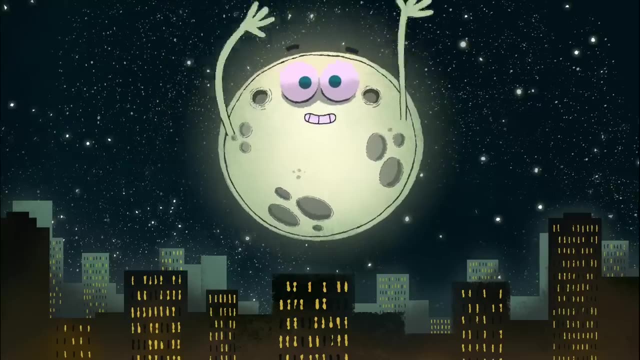 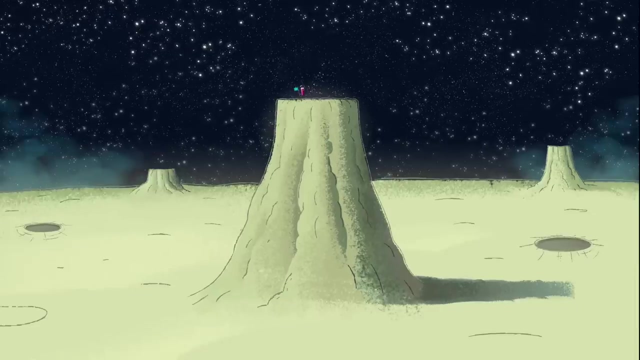 It's my time to shine. It's my time to shine. Both at night and at night we can see the moonshine. It's my time to shine. It's my time to shine. I'm planting this flag on the mountain I climbed. 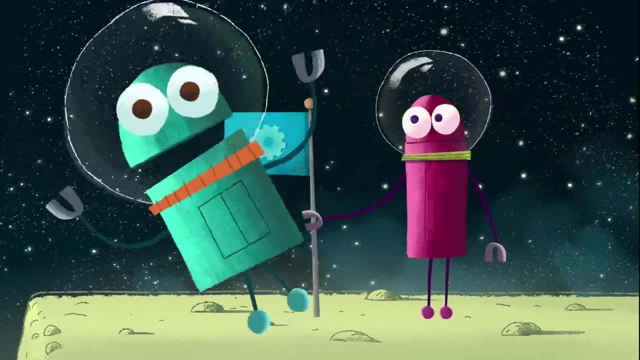 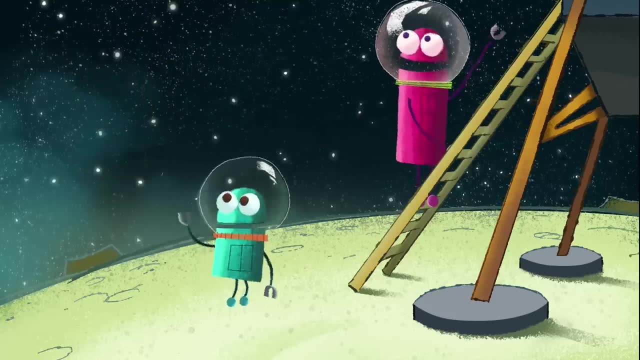 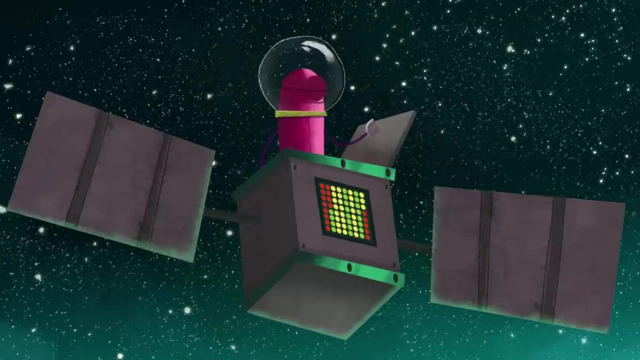 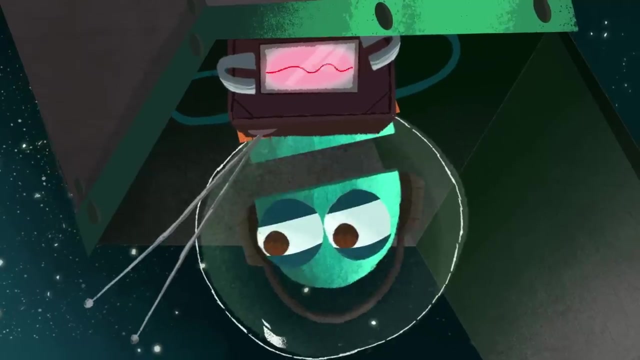 One small step for a story bot. One giant leap for story bot kind. One giant step for a story bot kind. One giant leap for story bot kind. Two giant steps for a story bot. We are currently orbiting planet earth. I'm picking up some noises. Sounds like cool music. 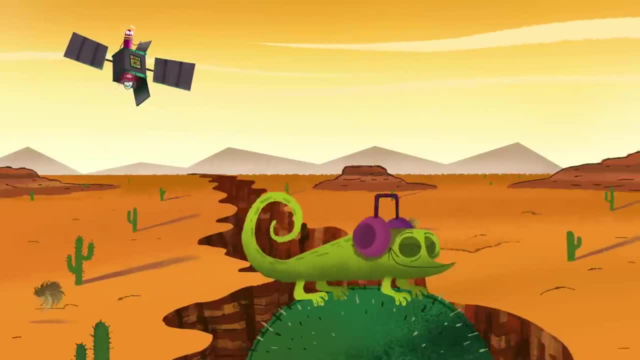 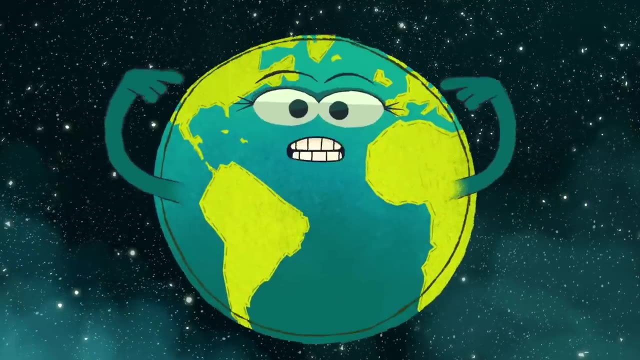 Such a beautiful, such a beautiful, such a beautiful, beautiful world. You're just playing with the music. You're just playing with the music. You're just playing with the music. I'm the Earth and for what it's worth, 25,000 miles is my girth. 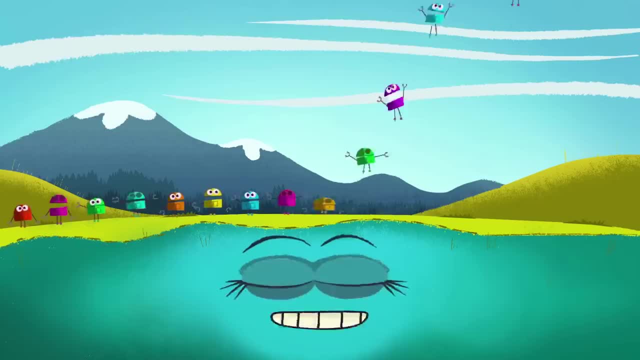 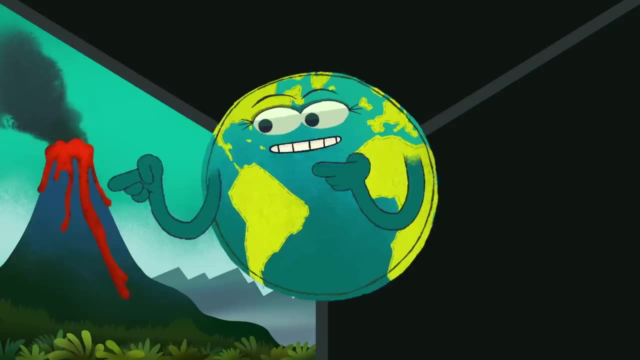 I've got more than 7 billion people living on me all across my amazing geography. Check out my mountains, valleys, trees so tall, and I got lakes, rivers and waterfalls, Volcanoes, craters, swamps with alligators. 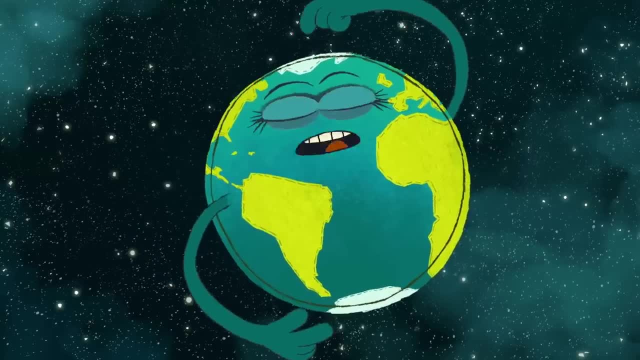 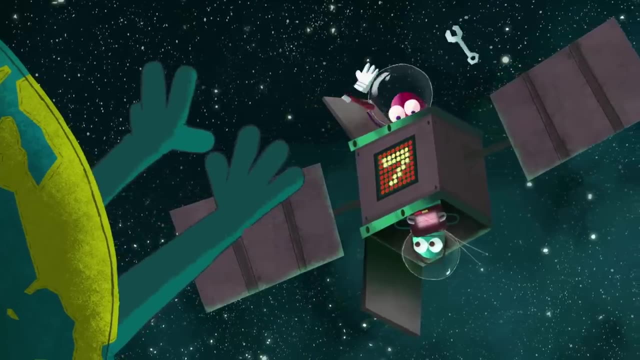 tropical islands at my equator, The North and South Poles have lots of ice. only polar bears say: This weather's nice, I've got so much land. yeah, I'm so immense. I got seven. seven different continents: North and South America, Europe, Asia, Africa, Antarctica and Australia. 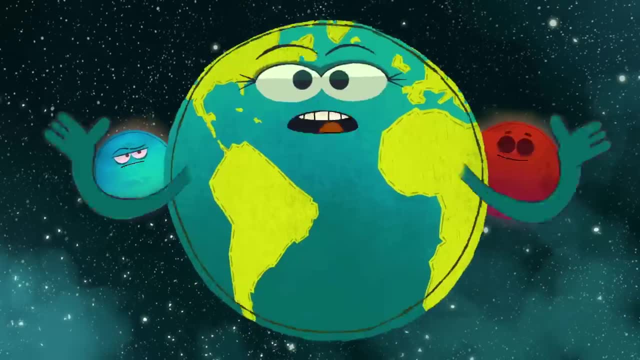 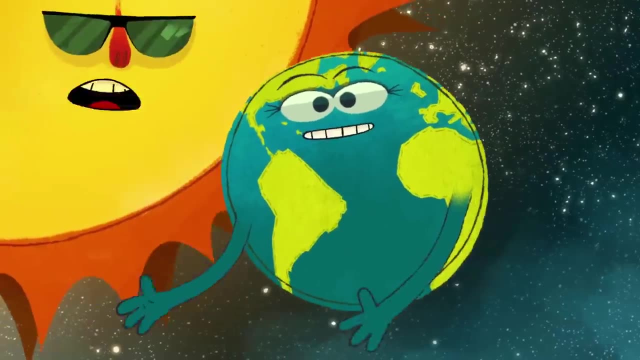 But the biggest thing everybody can see is that I got a lot of water all over me. I have oceans with lobsters, whales, otters. Three-quarters of me is covered in water. I orbit the sun- that's his line- and the moon orbits me. 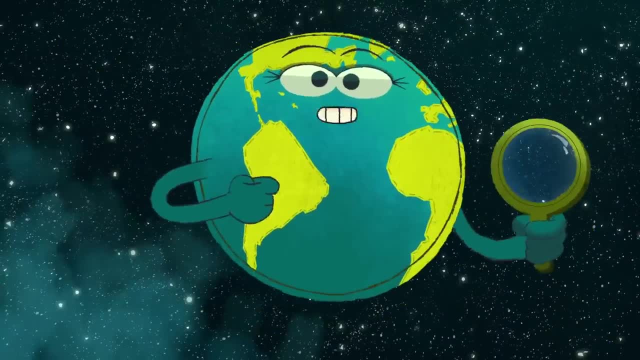 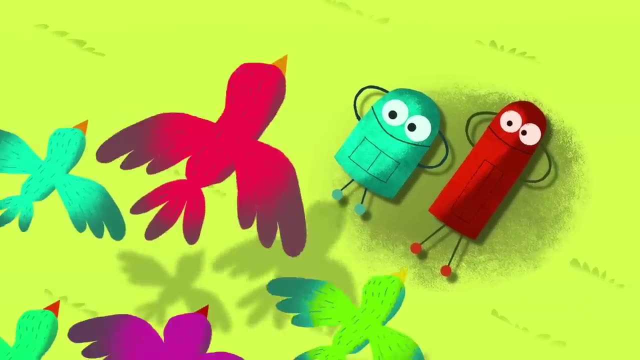 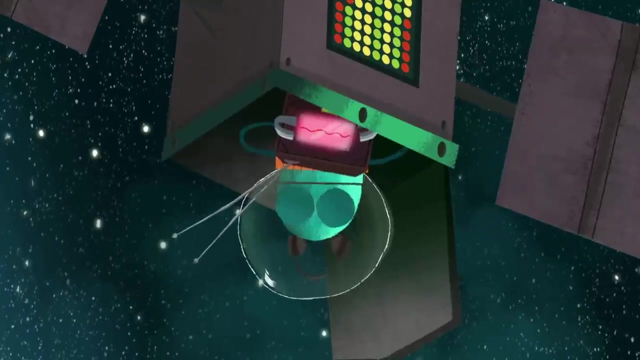 I'm filled with life, both big and small. the most beautiful planet of all, Such a beautiful, such a beautiful, such a beautiful, beautiful world. It is the home to every boy and girl. It's a beautiful, beautiful world. 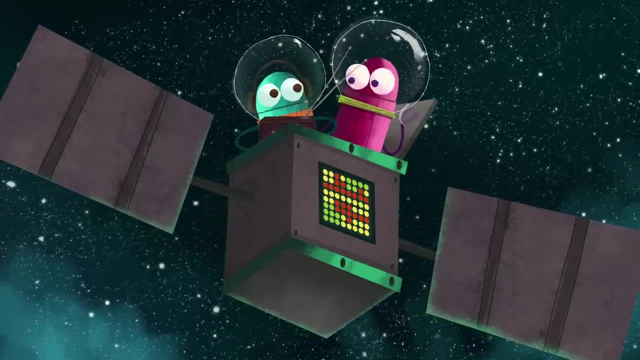 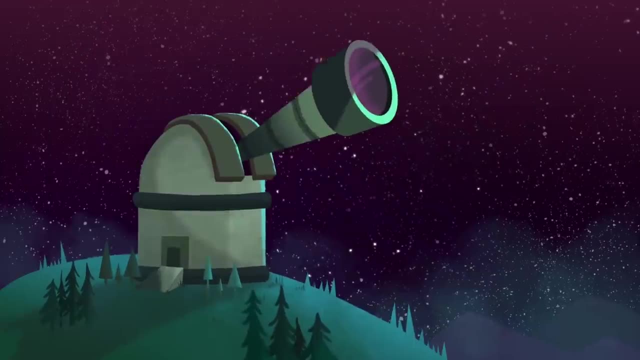 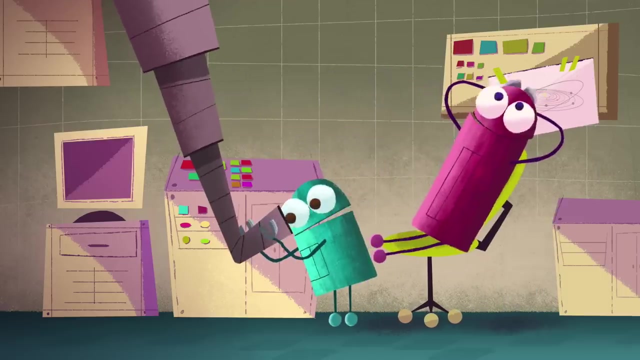 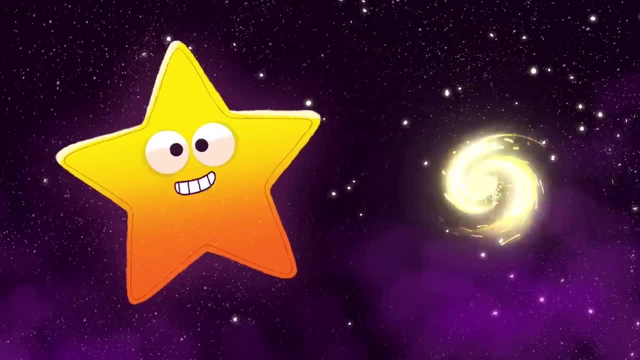 I'm a star. I'm a big, big star. I'm a star from afar. Yes, you are, And so am I. We are balls of hot gas that shine in the sky. There are trillions And trillions of us. 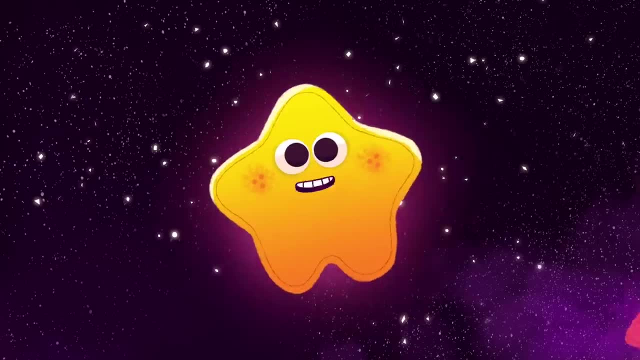 That's a lot. Even the sun is a star. The sun's so high. There are lots of other stars Like him And me And me And a bunch of us together form a galaxy. There's billions of galaxies, Lots of stars. 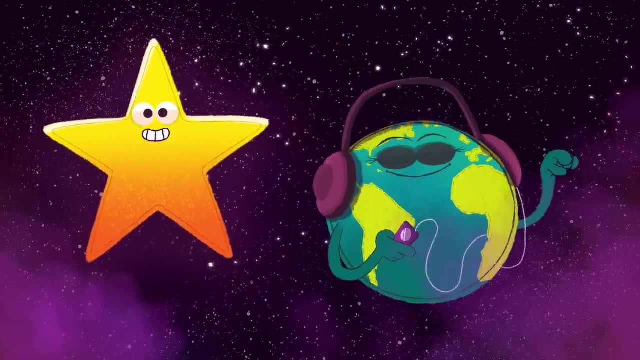 Understand. There's more stars in space than all of Earth's grains of sand. And from land, with your eye to the night sky display, You can see the Earth's galaxies, The Milky Way. The Milky Way Stars are different sizes And we can morph. 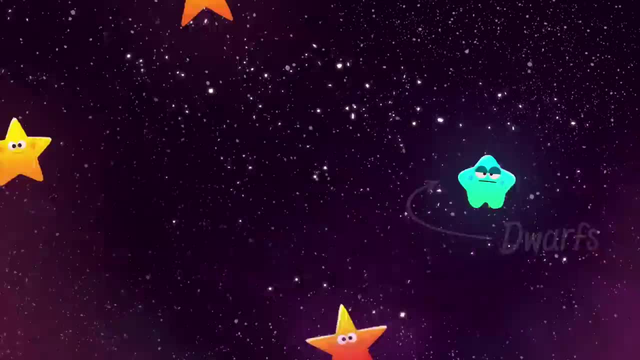 There are super giants, Giants Main sequence And dwarfs, And we form constellations Which are patterns of stars Before GPS. that's how you know where you are. We're the Big Dipper, We're the belt of Orion. 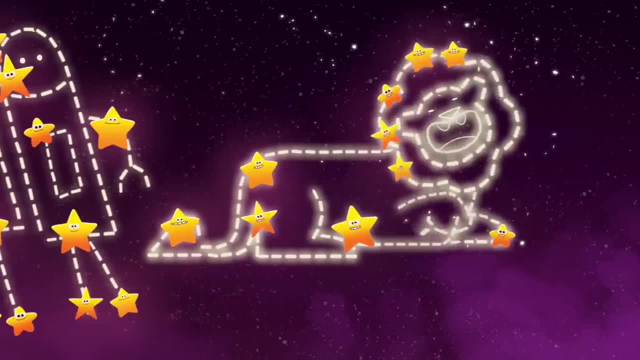 We're the Gemini twins. We're Leo the Lion. People think we twinkle, But that's not true. The light's just playing tricks when it shines on you. And shooting stars aren't stars. No, they're not. They're meteors burning up when they get too hot. 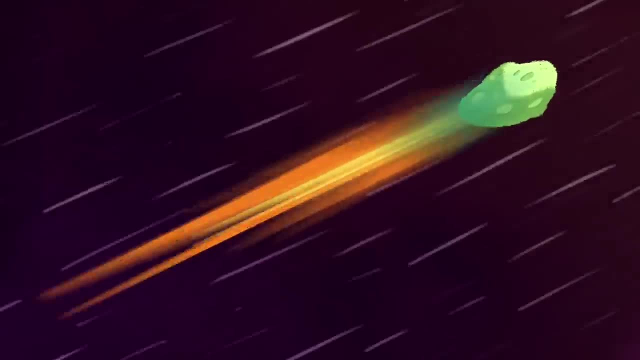 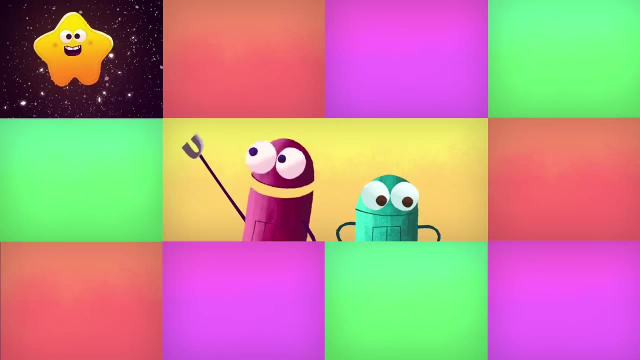 Wish upon a star Might come true Now, I hope. Look there's a star. Look there's a star. There's a star. Look up in the night sky, Or look through a telescope: There's a star. There's a star. 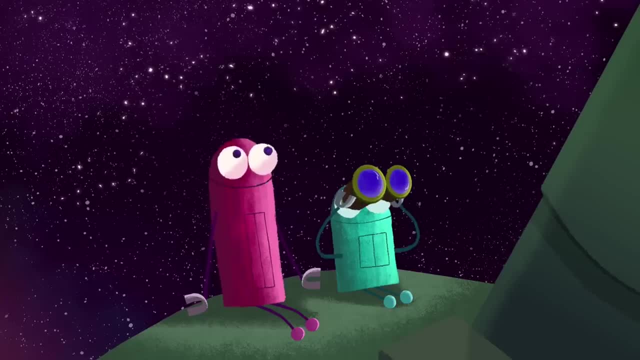 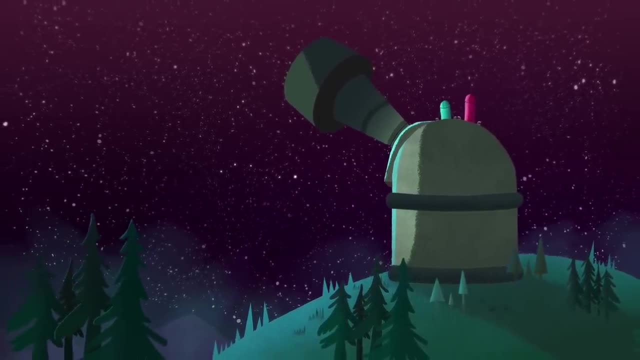 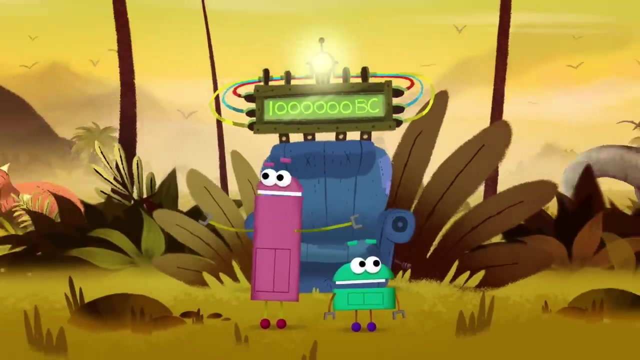 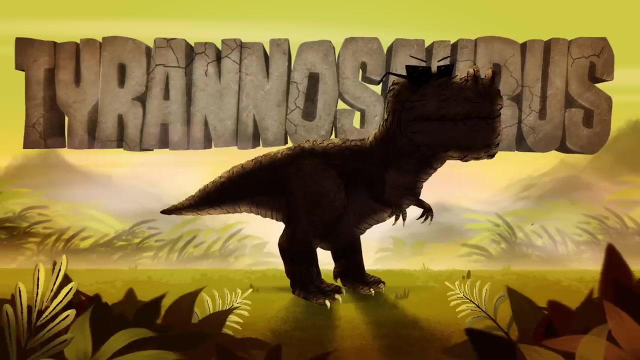 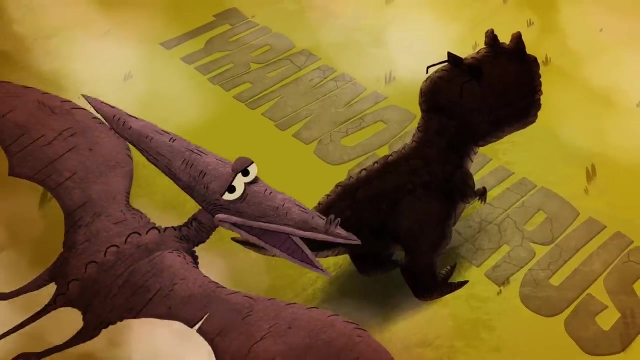 I'm not telling. Your time machine has taken us back 65.5 million years to the time of dinosaurs. This is where we hold school. Tyrannosaurus, That's the chorus. Tyrannosaurus, That's the chorus. Tyrannosaurus, That's the chorus. 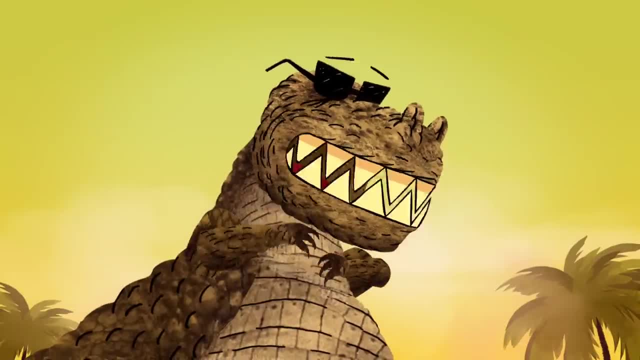 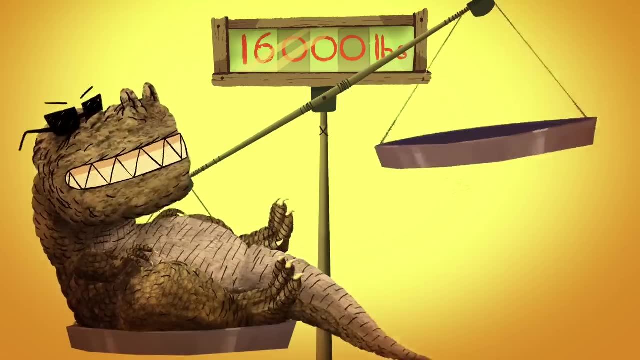 What's the chorus? Tyrannosaurus? Hey, I'm a Tyrannosaurus Rex, So big you gotta give me respect. I'm as tall as a house. you can't push me around Cause I'm heavy- 16,000 pounds. I got strong legs and a tail for support. 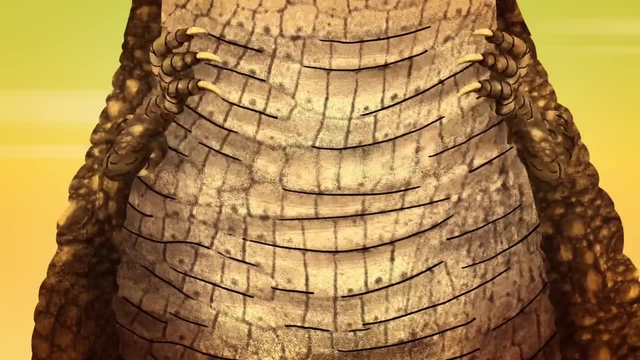 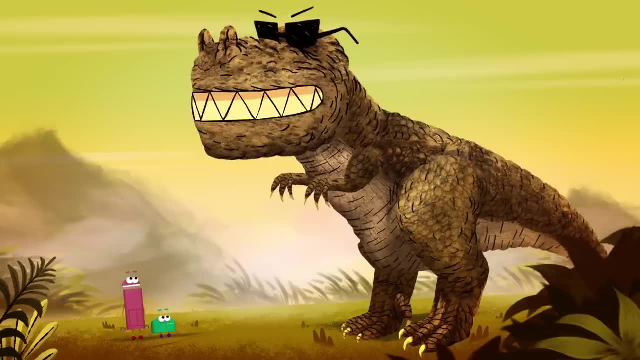 My tail is long, but my arms are short. See, my arms can't touch And, what's even more, I'm not even sure what to use them for. But my mouth is big and my teeth are scary. Over 50 teeth- how sharp are they? 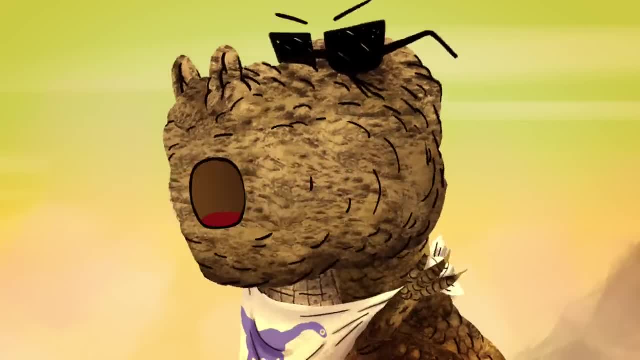 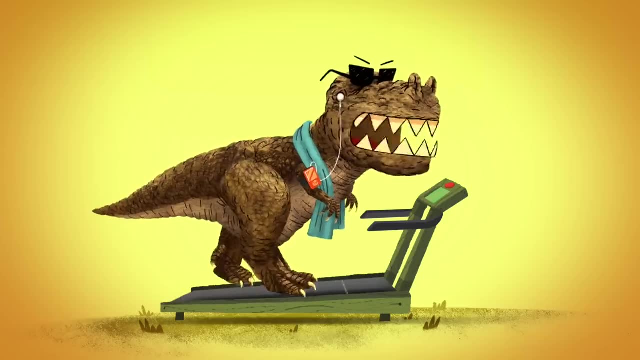 Very big, long teeth make it easy to eat And I'm a carnivore, which means I eat meat. I got a good sense of smell, hearing and sight So I can go hunting both the day and the night. Yeah, I'm not very fast, but that don't mean a thing. 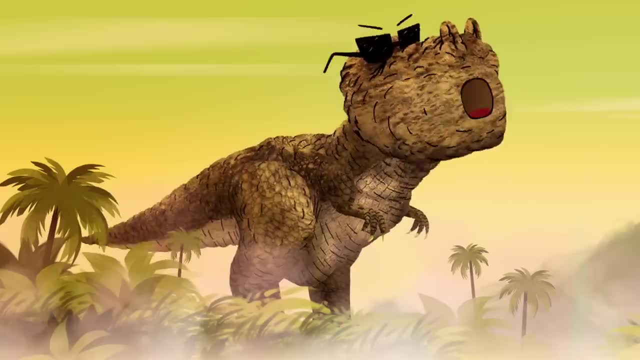 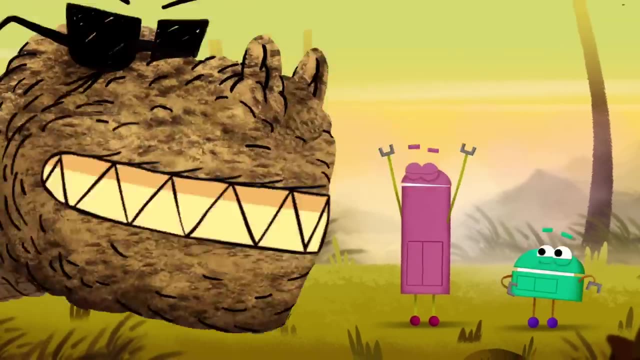 I'm the king of the dinos. it's good to be king Tyrannosaurus. That's the chorus Tyrannosaurus. That's the chorus Tyrannosaurus. That is the chorus. What's the chorus Tyrannosaurus? Wow, his teeth are really big. 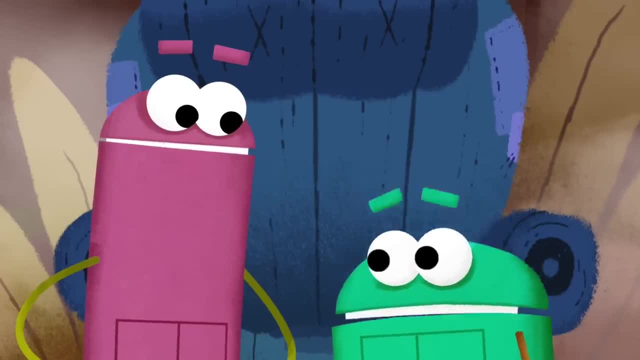 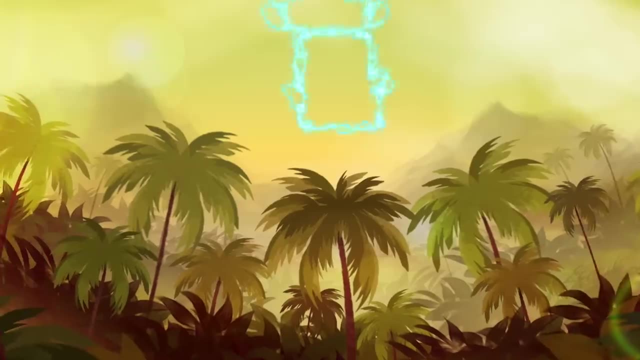 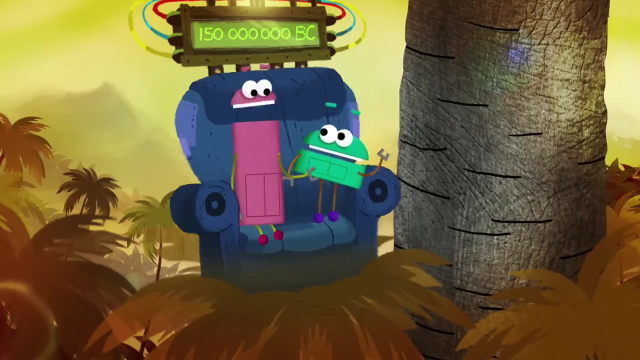 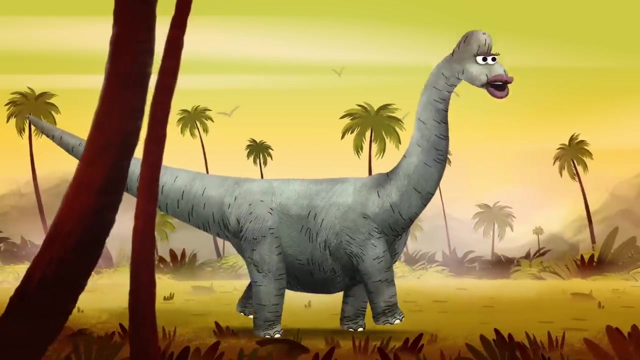 I'm just glad he eats meat and not storybots. We are now in the Jurassic period. Look at that tall tree. That's not a tree. My neck's so long And my neck's so strong- I can bounce my head up and down While I'm rapping my song. 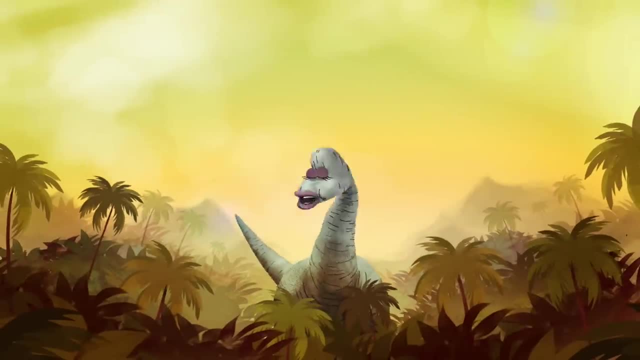 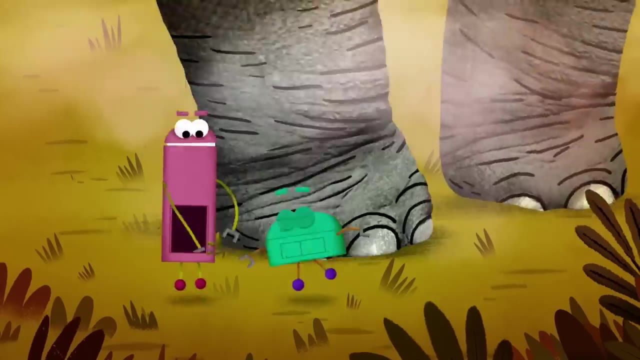 What's up? I'm an Apatosaurus. I'm the biggest thing in this whole forest. Got a long, long, long, long neck. Don't get it twisted. I'm one of the biggest animals that ever existed. When I walk, it sounds like thunder. 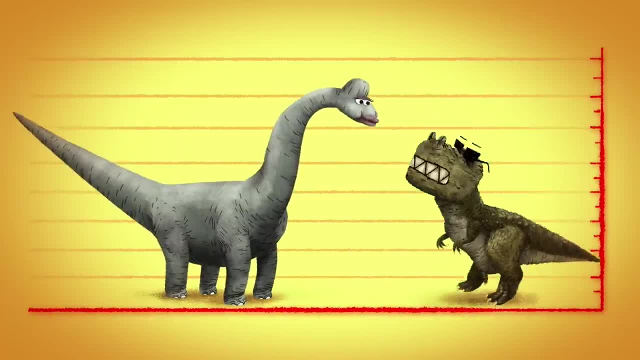 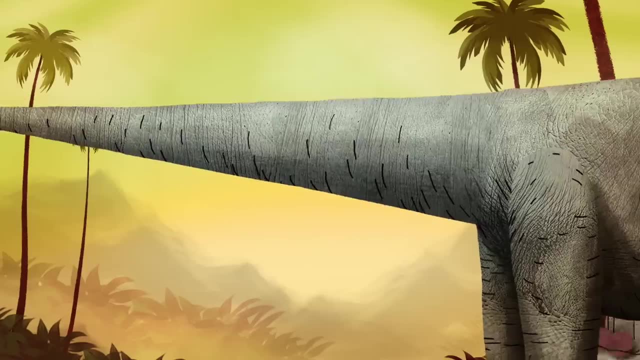 Is there anyone bigger than me, I wonder? T-Rex Triceratops Velociraptor, You can squash us with your jaw, That's right. I'm the biggest. Nobody wants to fight. Nobody's at my height Or in my eyesight. 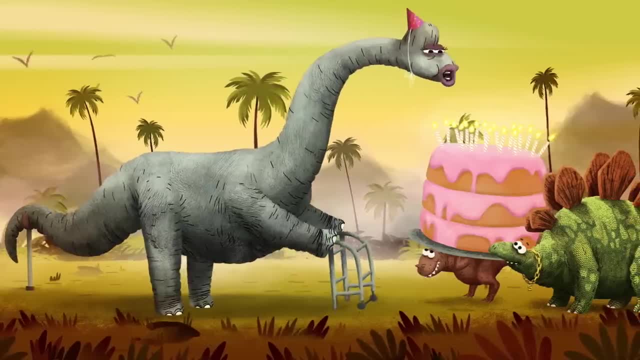 I can whip my long tail to scare others away. I can live to be a hundred years old and grow up to be a man. I can live to be a hundred years old and grow up to be a man. I can live to be a hundred years old. 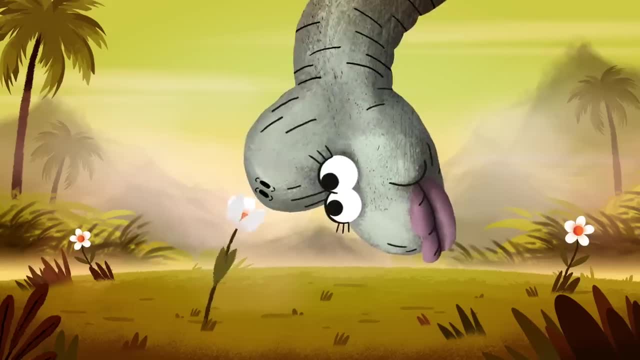 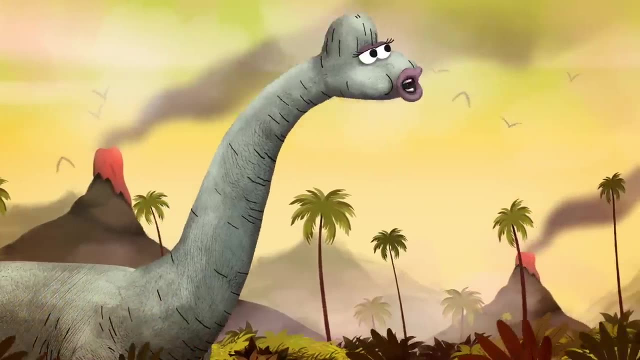 I eat plants and eat rocks to help me digest. Got nostrils on my head, big heart inside my chest, But the part that's best gotta give me respect, Got a long, long, long, long, long, long neck, My neck's so long. 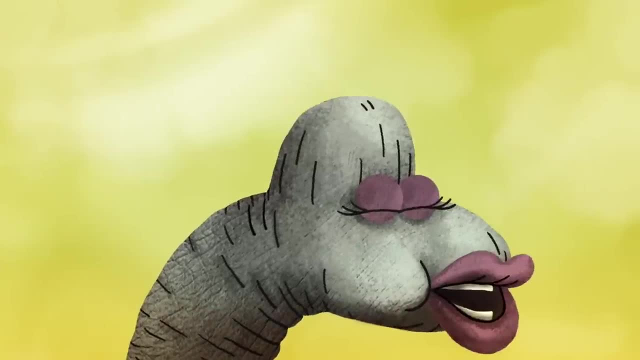 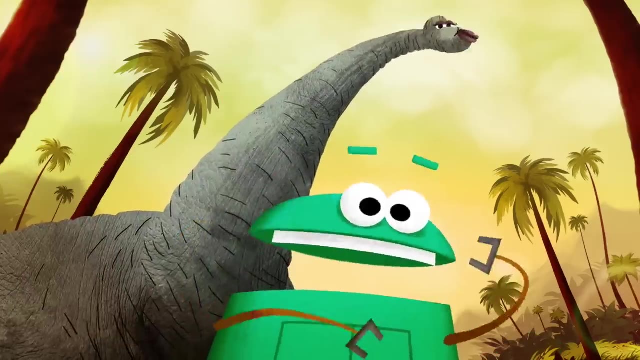 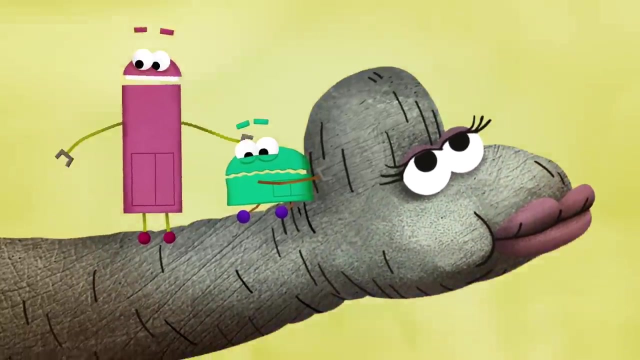 And my neck's so strong I can bounce my head up and down While I'm rapping my song. Her neck is long And her neck is strong. We can bounce our heads up and down While we're rapping this song. Dinosaur Elevator. Dinosaur Elevator. 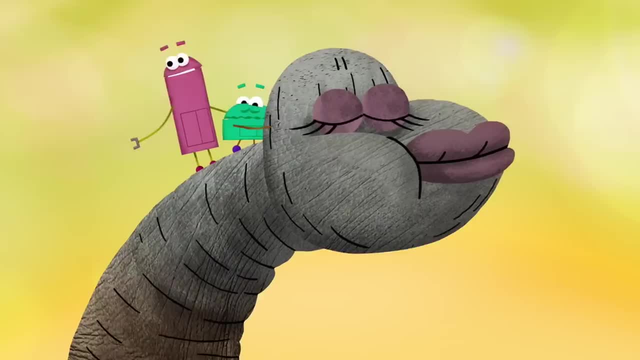 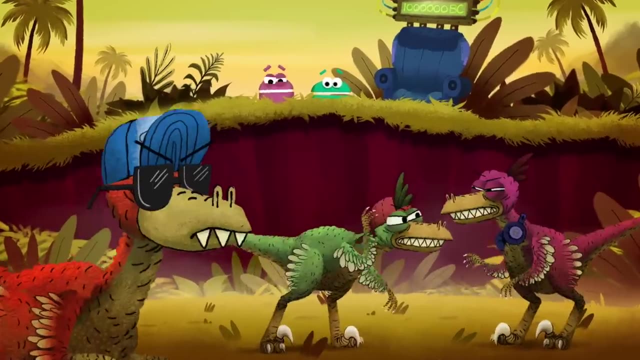 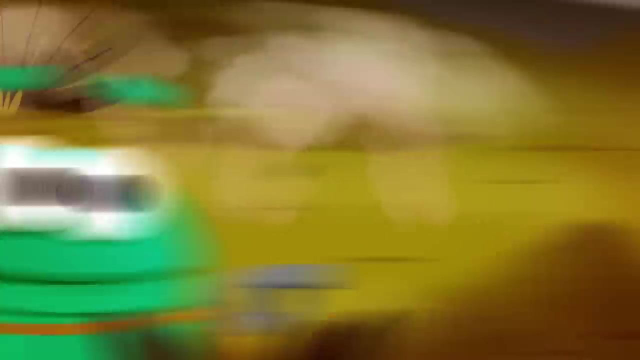 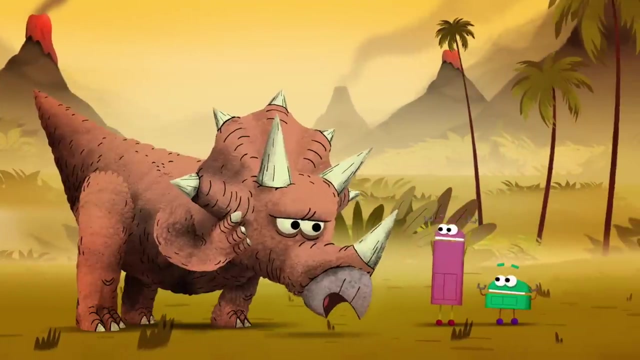 Wake up. Good thing we are not afraid of heights. I hate park ourselves. I wonder if there are friendly dinosaurs. That one looks pretty cool. One, two, three, Check out Mars. One, two, three, Check out Mars. I'm a triceratops All up in this place. 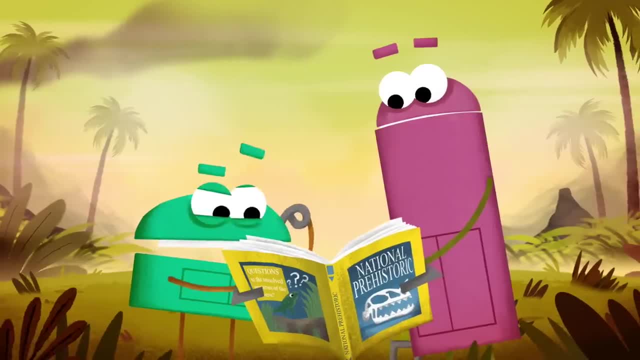 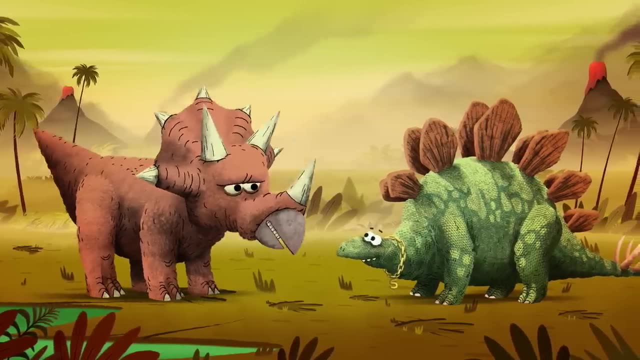 Triceratops Means three-horned face. What do I use them? for? Scientists debate, Maybe for defense Or to find a mate, But I love my horns, Three up on my grill. I'm also really special Because I have a frill- A frill. 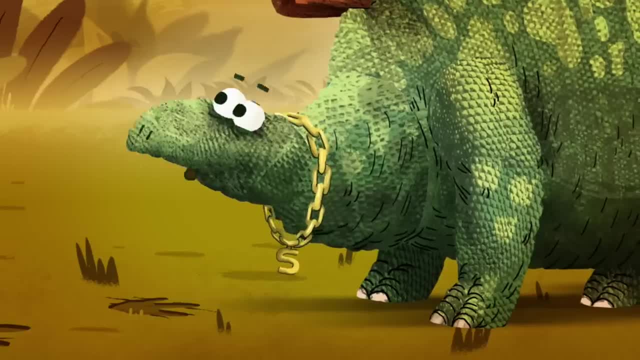 Yeah, a frill. You heard what I said. It's a plate of bone on top of my head. Cool Sorta, looks like a crown. I'm a king of a kind. Hey, I'm the king of the dinosaurs and I'm hungry. Never mind, The T-Rex would eat me if he had the chance. 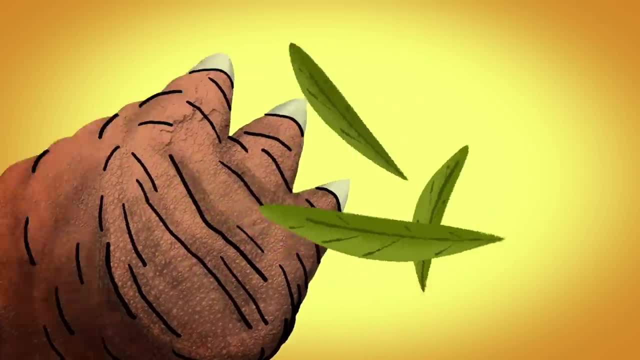 But I'm a herbivore. I only eat plants. got hundreds of teeth To chew my veggie food. Got a small pointy tail, But I'm a big dude. I move pretty slow and got hooves on my feet. But check it, cuz I'm a herbivore. 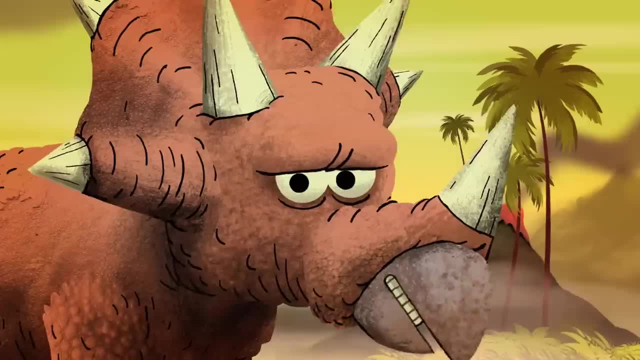 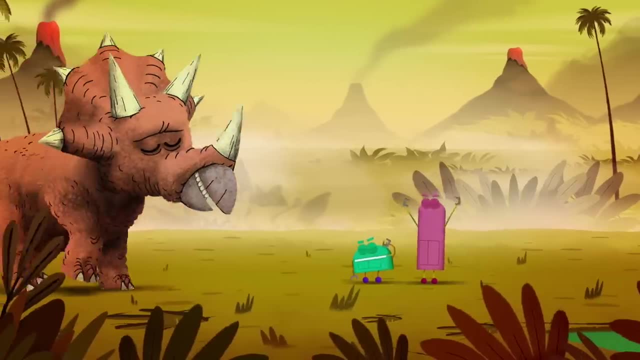 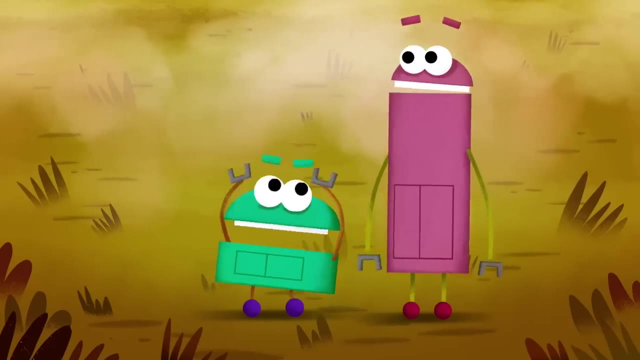 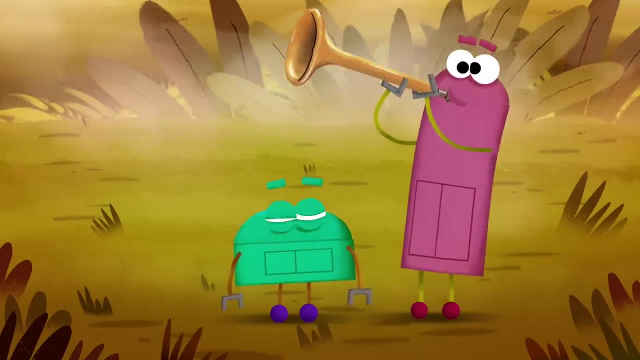 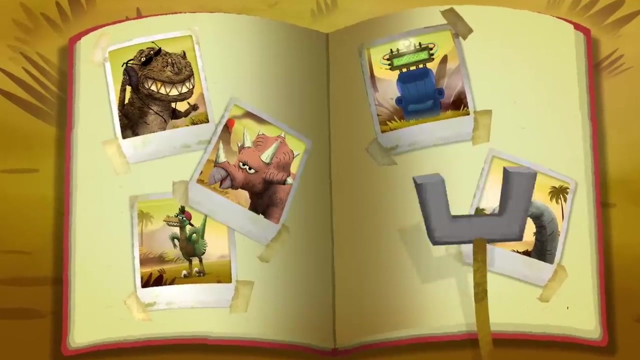 These horns are pretty sweet, right. One, two, three. Check out my horns. One, two, three. Check out my horns. One, two, three. Check out his horns. One, two, three. I wish I had a horn. Here you go. We've seen some pretty cool dinosaurs so far. 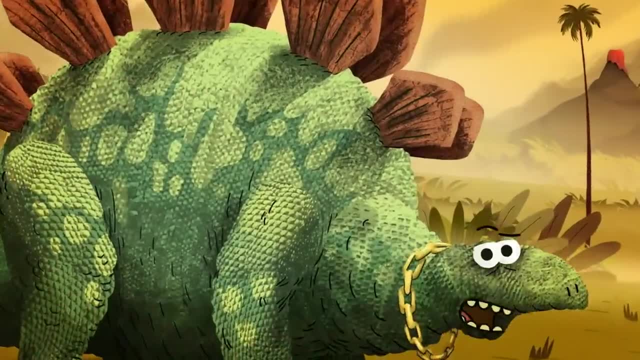 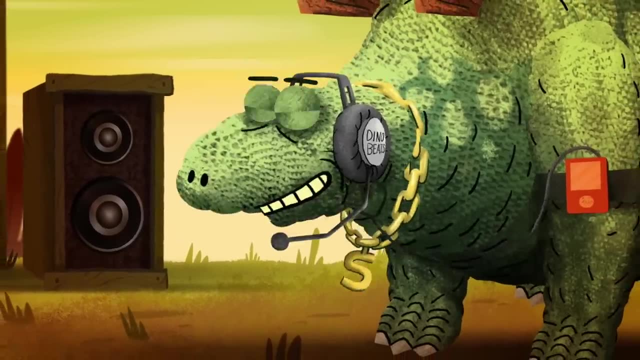 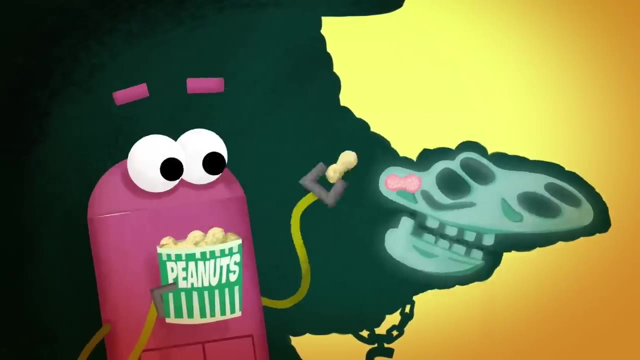 That one has things all over his back. Okay, My sack is covered in plates, My tail is covered in spikes, And that's why I look great. When I'm rocking the bike, I'm like I'm a stegosaurus, What's up yo? I may have a small brain and move pretty slow. 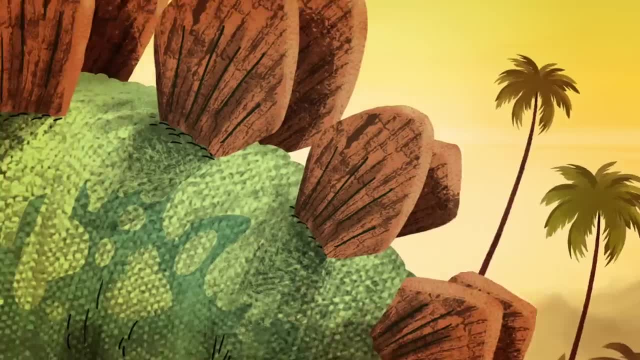 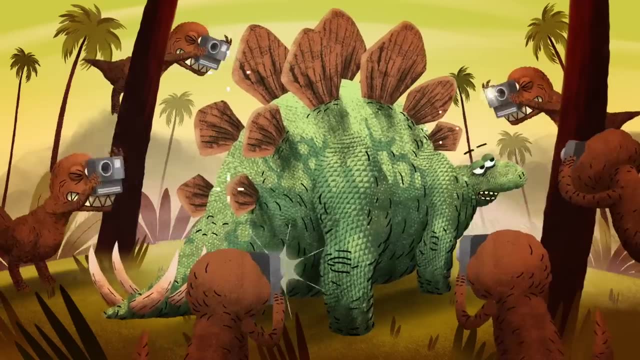 But I've got a spiky tail. I can swing and attack And I've got all these plates on top of me, these plates on top of my back- Not plates for food, dude, They're part of my body. They make me attractive. I'm kind of a hottie. I can use my plates for attractive mates, So we can go out. 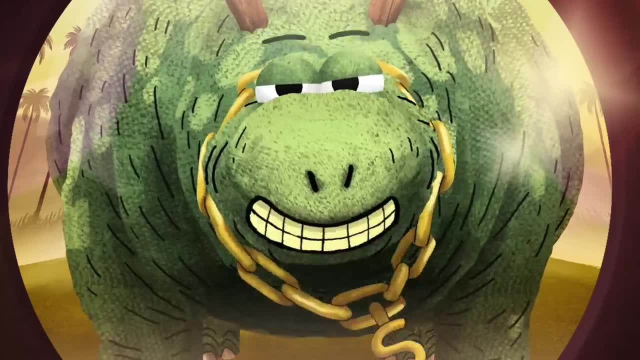 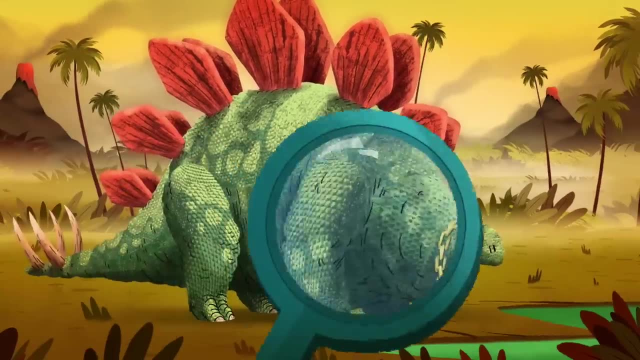 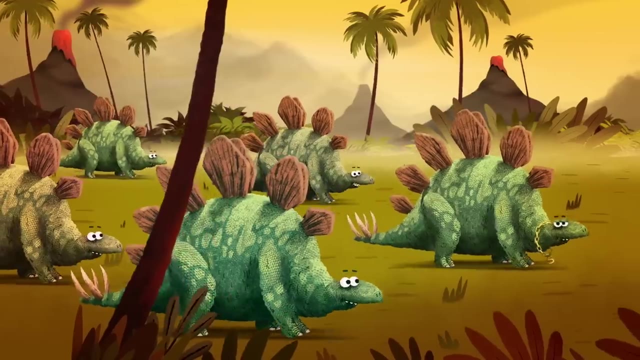 on stegosaurus dates. I also use my plates to generate heat and scare away predators: Retreat. My plates are so cool I can make them turn red. I got a huge body and a very small head And I got big cheeks for food I can store, But I only eat plants because I'm an herbivore. I got lots. 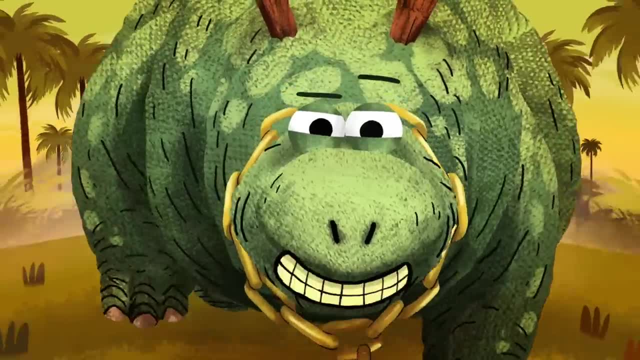 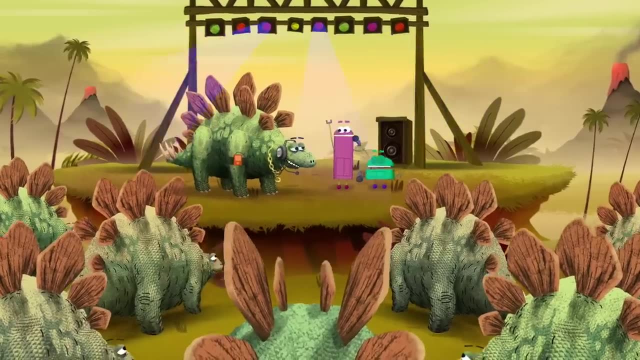 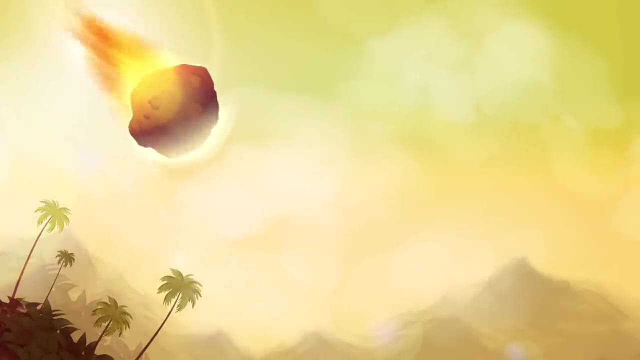 of friends and we're moving to herd And we all are super good looking. Word: Our backs are covered in plates, Our tails are covered in spikes And that's why they look great When they're rocking the mic. Uh-oh, An asteroid is approaching. Let's go back in the time machine. 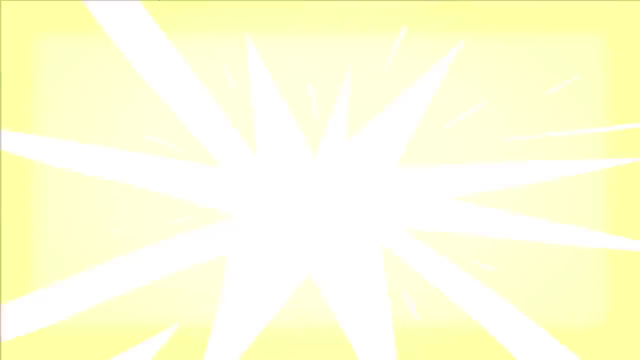 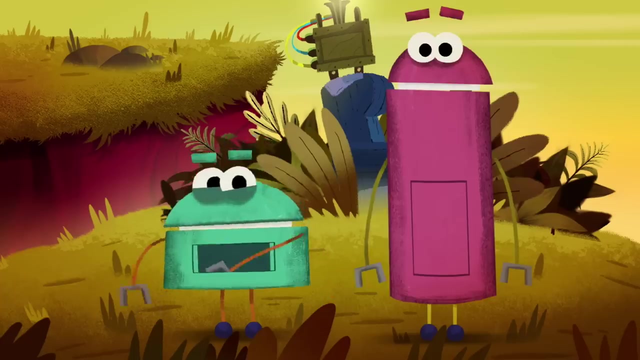 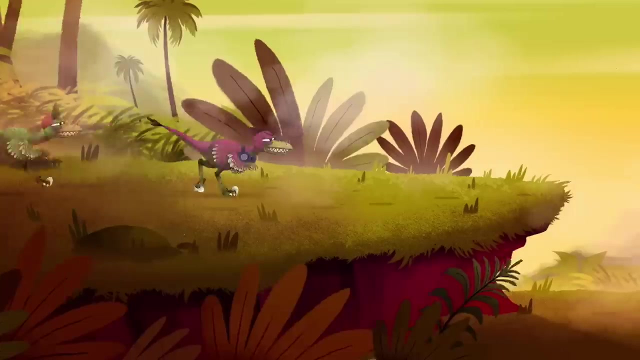 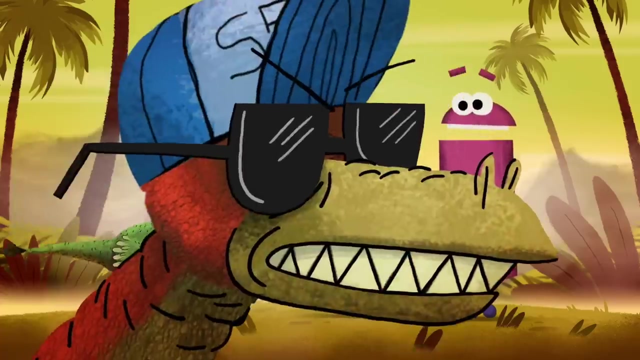 We are now In the Cretaceous period. Looks like there's some dinosaurs approaching Fast, Velociraptors velocirapping. When we run up, who knows what'll happen? Velociraptors velocirapping, Don't get too close. the teeth will start snapping When it comes to dinosaurs. 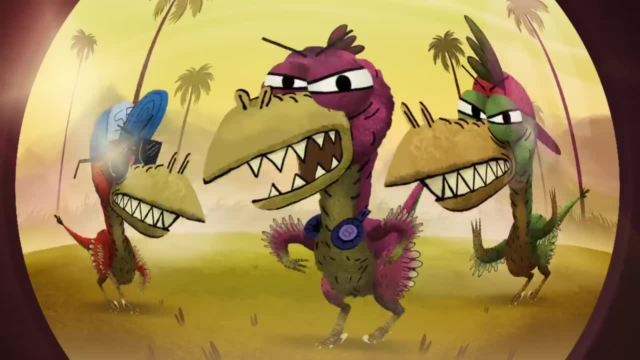 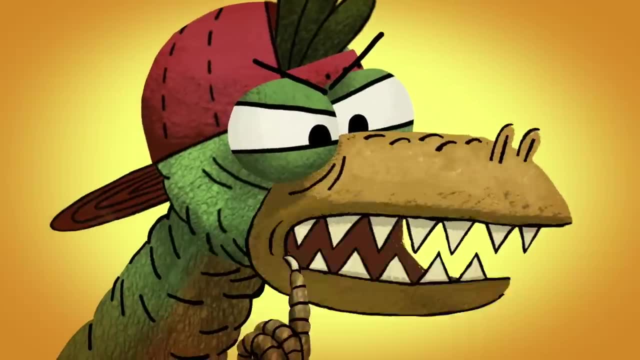 we are small, Six feet long and three feet tall, But our size doesn't matter at all. We're quick and speedy when it's time to pull Long, flat snout, with a real strong jaw, Jagged teeth and a real sharp paw. When we eat food, we like it raw: Shimmy, shimmy, I am shimmy, Are you? 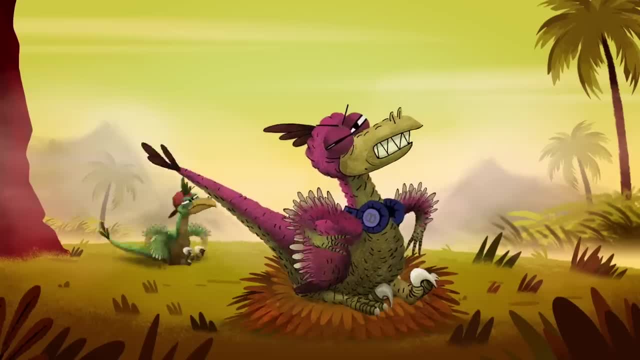 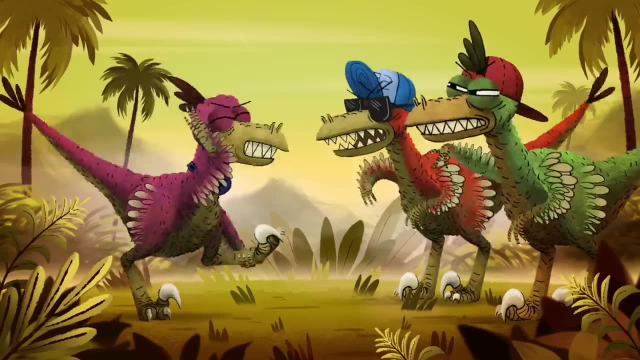 shimmy at all. We look like birds, you may have guessed. We lay eggs inside a nest. We've got feathers, so we stay well dressed. I'm the king of the dinos. even I'm impressed. Long, strong legs with lots of power, Running 24 miles per hour. We don't want to eat that.